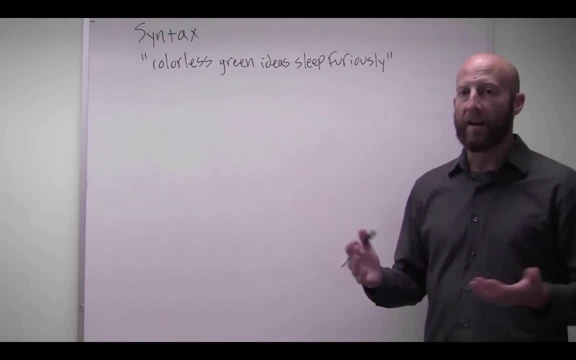 basically to illustrate the importance of syntax. So you might look at this and immediately recognize that there's something wrong. It doesn't make any sense or very little sense, But there's also something right about it. It's a perfectly well-formed sentence in English. 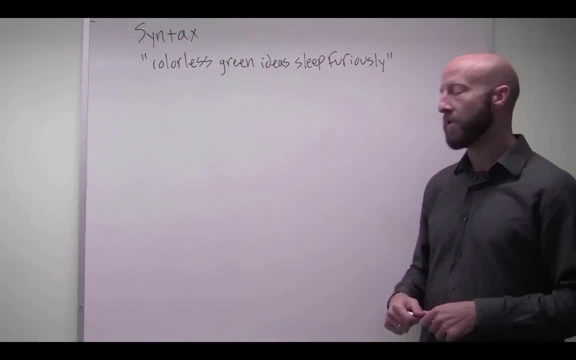 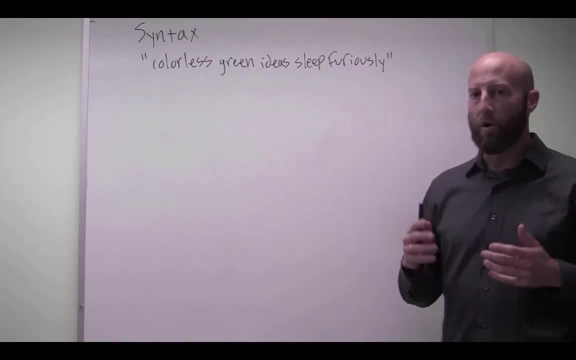 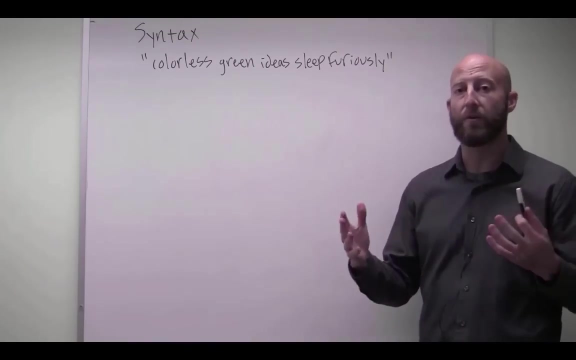 syntactically, That is, you have two adverb or two adjectives preceding a noun and you have an adverb coming after it. So all of those elements are in the right order. It's a perfectly well-formed sentence, and it therefore illustrates that syntax is a real thing, even. 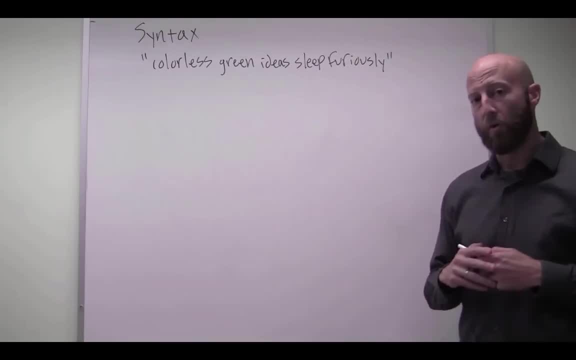 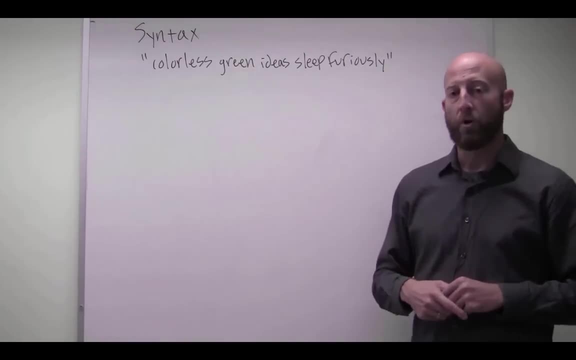 if it doesn't make any sense semantically. So in this video, we're going to be talking about three things. We're going to talk about lexical categories, otherwise known as parts of speech, which will be important for understanding phrase structure, rules, which, in turn, will be important for understanding how to use them. 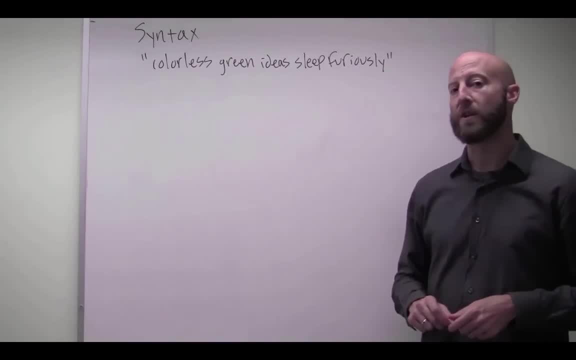 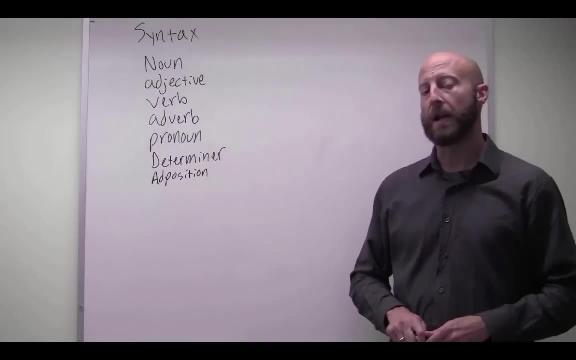 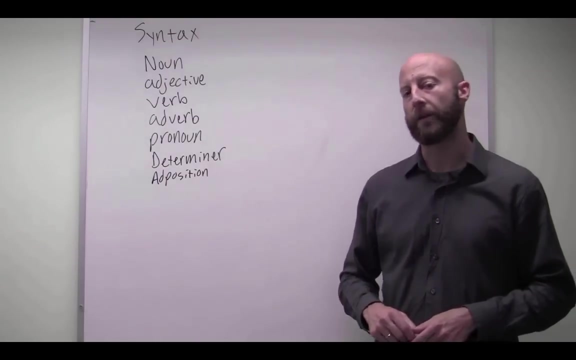 So let's get started. First let's talk about lexical categories, which is really just a fancy way of saying parts of speech. But get in the habit of saying lexical category. I think it makes a little bit more sense than parts of speech, which is a phrase you probably remember from English. 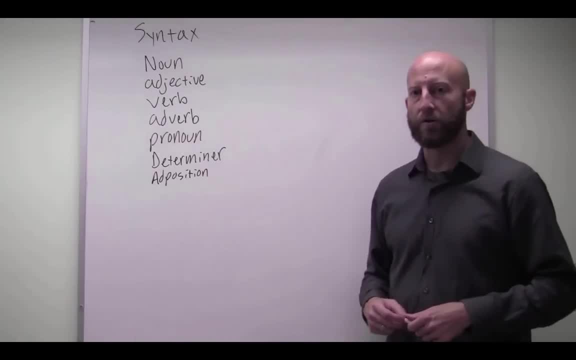 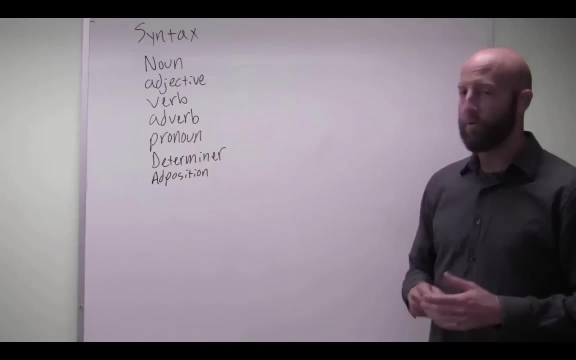 class. Anyway, when we're talking about drawing tree structures, it's really important to know these lexical categories and you probably know most, if not all of them. But anyway, let's just briefly review what they are. So a noun- typically it's some sort of person, place or thing As a subject. in English, 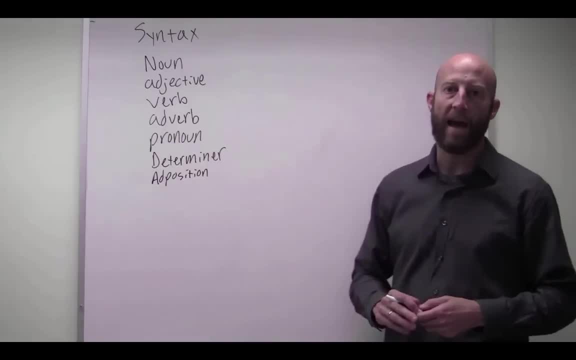 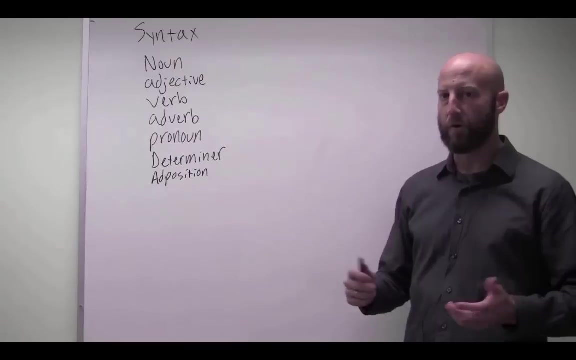 they're nouns. They pretty much have to be nouns. So cat, house, swimming pool, person, place or thing, Adjectives are always going with nouns, because adjectives describe or modify nouns. Red, big, huge, that sort of thing Verbs are the action in the sentence. 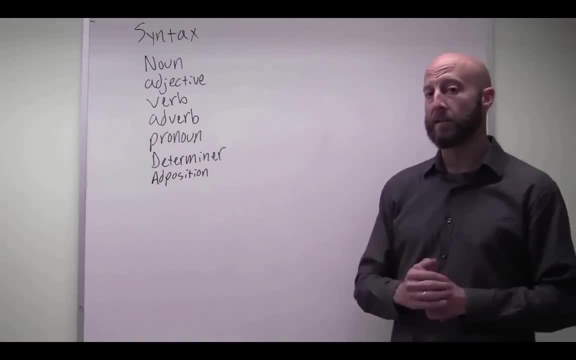 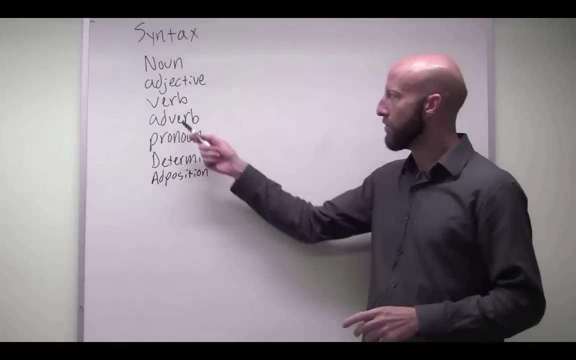 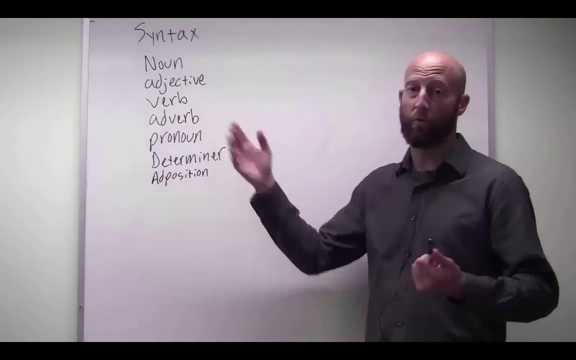 so it's denoting some sort of action event. so swim live is. those are all instances of verbs. adverbs go with verbs, just like adjectives always go with nouns, and it's easy to forget that, but adverb has the word verb in it, so use that as a mnemonic device to remember. 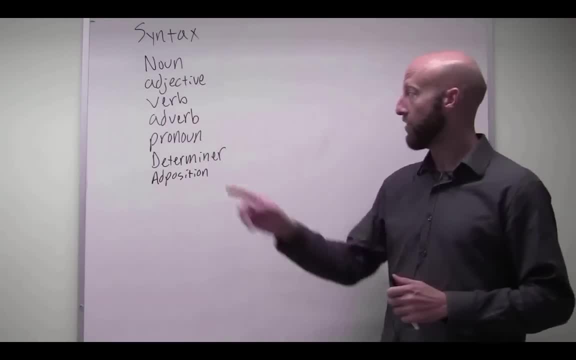 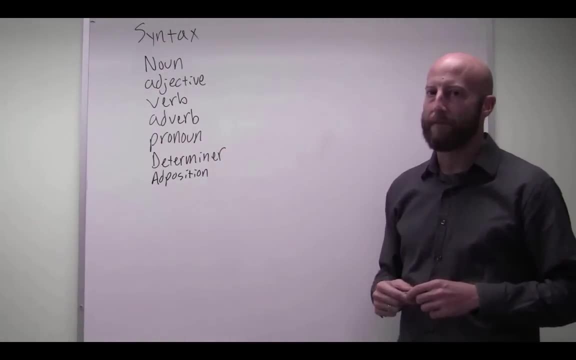 adverbs are always describing verbs, just like adjectives are always describing nouns. in English, you almost always know that you're dealing with an adverb, because most of the time, the word will end in ly. there are some exceptions, though, like friendly or ugly. those are actually adjectives because they always 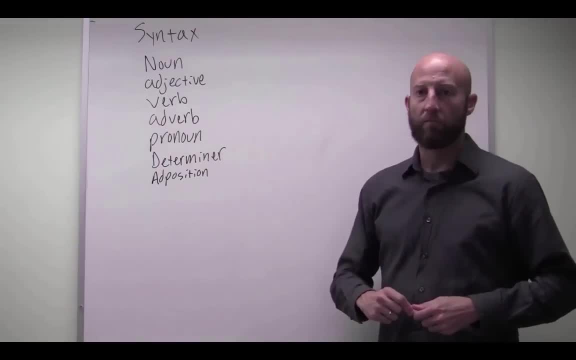 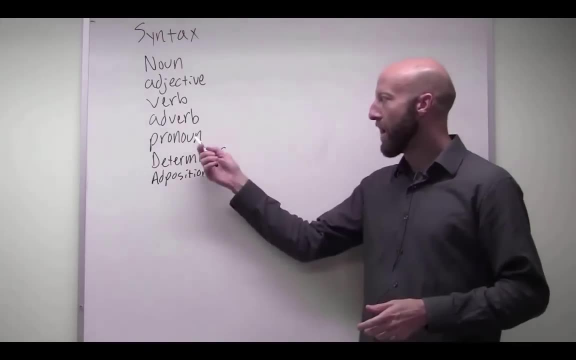 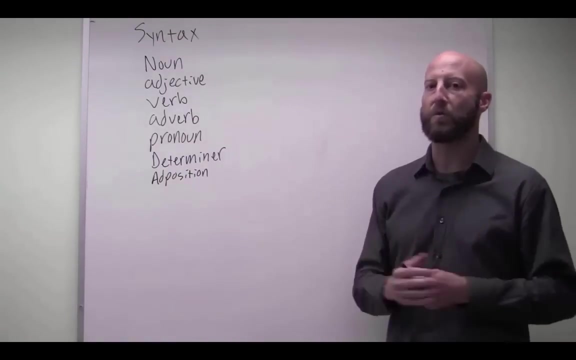 describe nouns, but things like quickly, slowly, those describe verbs and as such we'd want to call them adverbs. pronouns are very similar to nouns. they behave almost the same exact way as nouns in English, but I'm treating them as two different things, just to kind of get you used to. 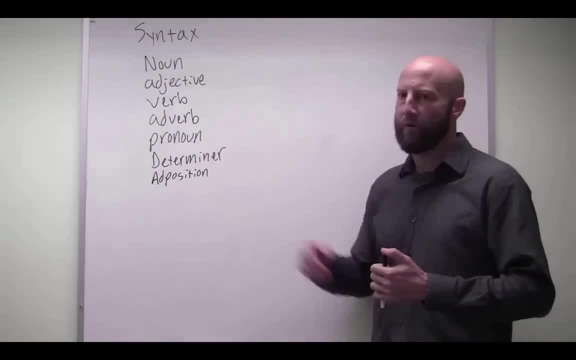 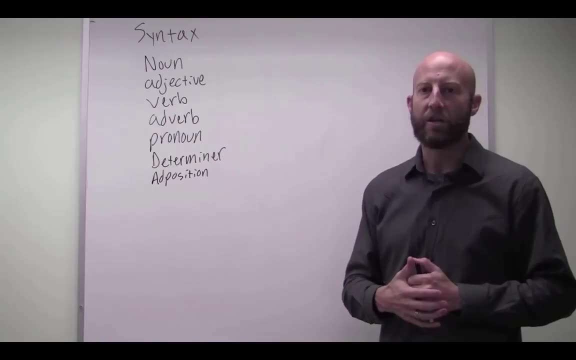 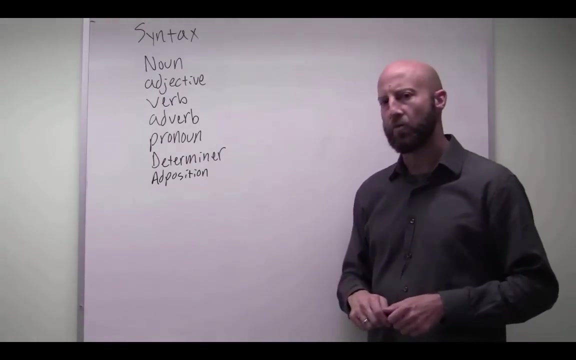 this technical difference between the two. so pronouns are always kind of pointing to someone or something, like that or not, that actually you, he, she it, so it's representing a person or a thing. determiner is the next one, and I want to call your attention to this one because your book doesn't cover determiners. it. 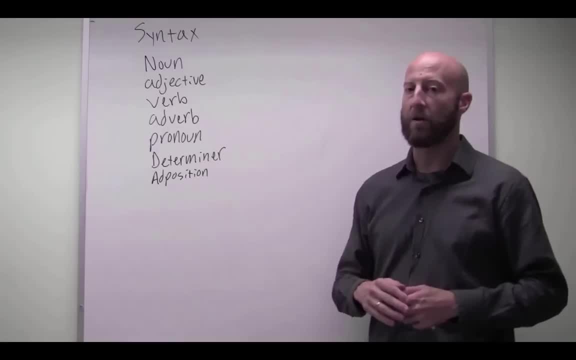 just mentions articles a and or the articles and determiners in this class pretty much use them interchangeably because we're not going into any great detail with either one of them. but technically there is a difference. articles are part of a bitter bigger category called determiners. determiners- 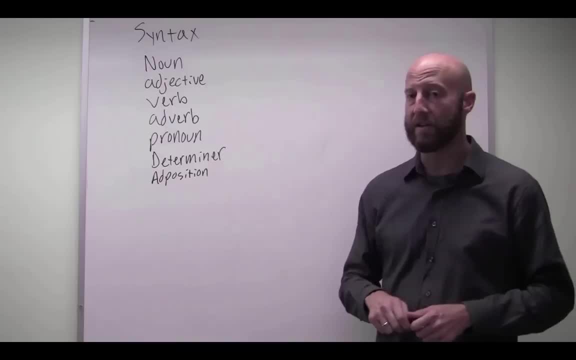 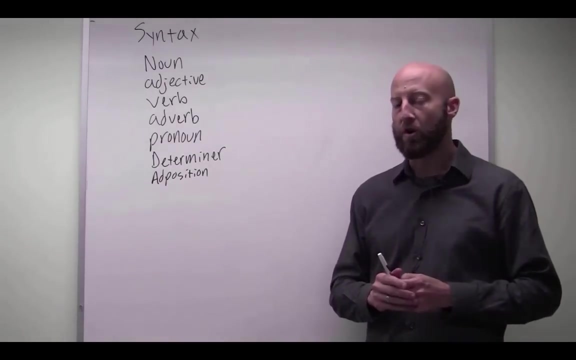 also include things like possessive pronouns like his, her, your, demonstrative, like this, that these, those quantifiers like one, some, many, that sort of thing. so maybe get used to the distinction between articles and determiners, but in this class you can use the two interchangeably. it's totally fine this. 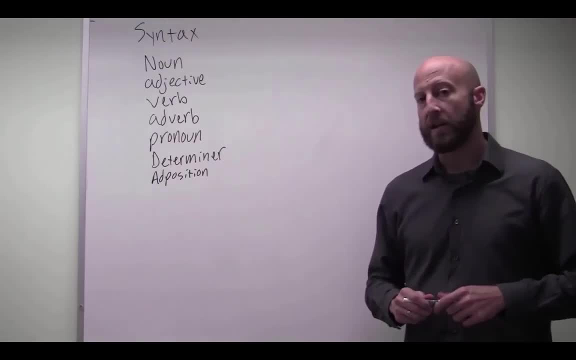 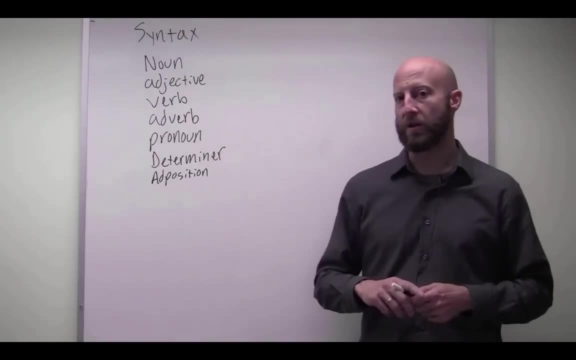 last one maybe you've never heard before. it's called an ad position. it includes something that you've definitely heard before: a preposition. a preposition is sort of asserting the trajectory towards something like to into the house or from as in, from the pool, near as in near the mountain. so it has something to do in. 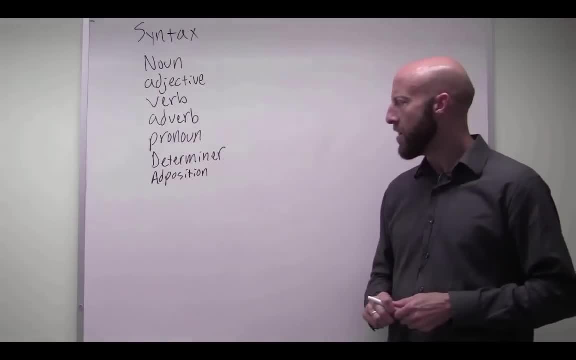 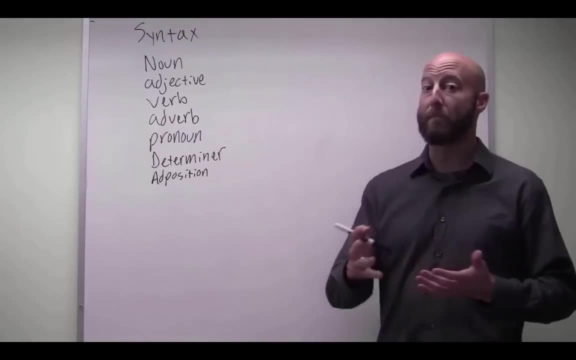 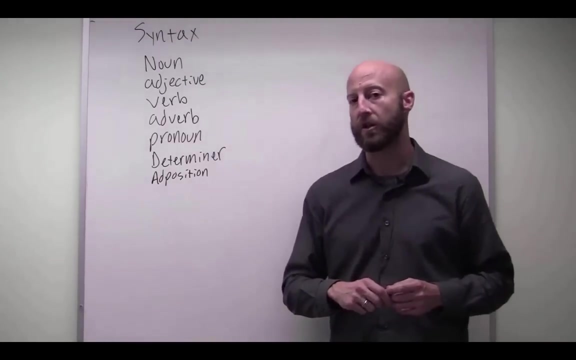 English with the direction or location of something. but what makes those prepositions in English is that they precede that object compliment. they always go before it and preposition pre position. but some languages do the opposite. they do what's called post positions, like Japanese, Turkish or. 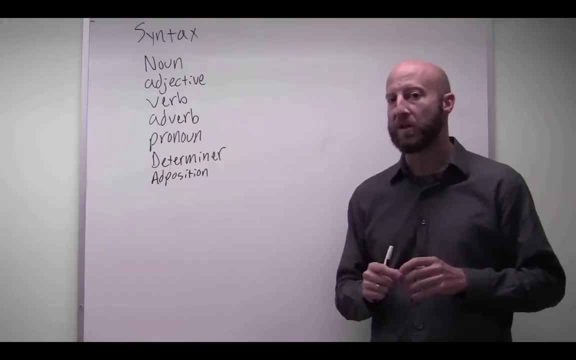 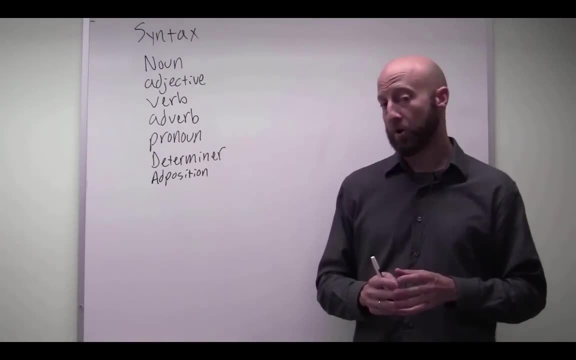 catch you up. they use not prepositions but post positions, so the thing comes after the object or compliment, and both of those together. prepositions and post positions are part of a bigger category ad positions- knowing these is going to be really in order to draw accurate tree diagrams. 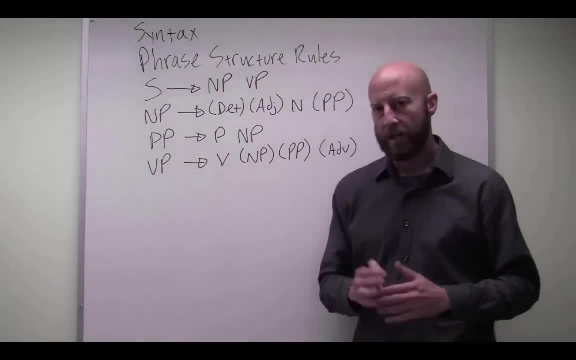 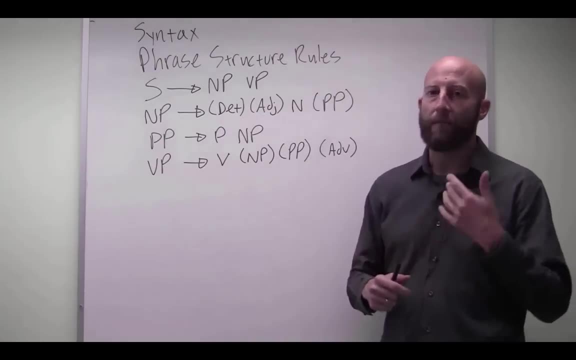 All right, so now let's talk about phrase structure rules. This is where we can start to see how languages distinguish themselves from one another, Because, while a lot of different languages have nouns and verbs and adjectives and adverbs, it's the phrase structure rules that basically tell you how you can combine those elements. 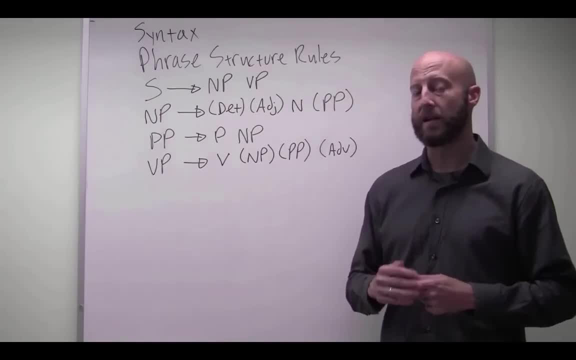 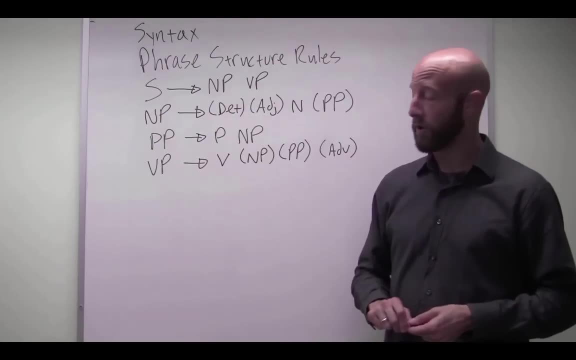 and which orders are acceptable to form sentences in that language. So here we have phrase structure rules, But keep in mind that these are the phrase structure rules for English, So let me just break down what this code means. So the first one is S arrow NPVP. 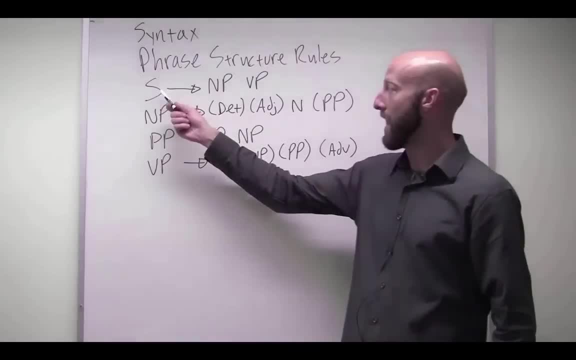 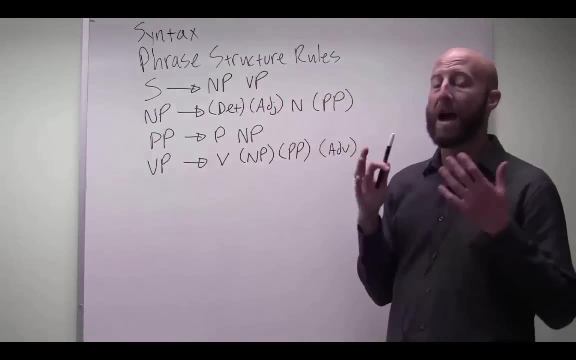 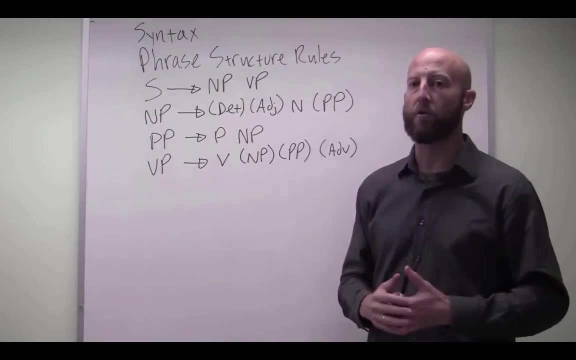 That, basically, is shorthand that linguists use to say that an S or a sentence consists of a noun phrase and a verb phrase. You have to have both the noun phrase followed by the verb phrase in that order in English to have a well-formed, acceptable sentence. 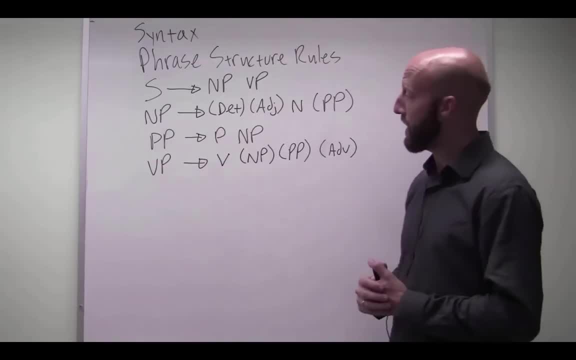 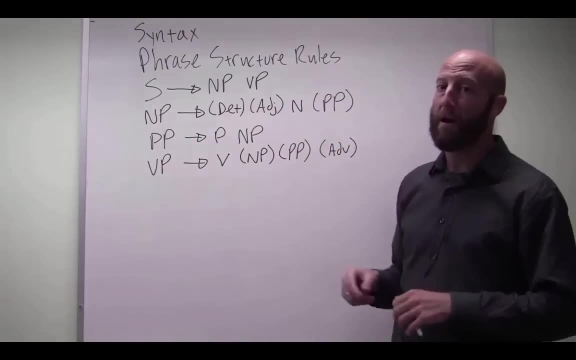 So what goes into a noun phrase, you may ask. Well, a noun phrase consists of a noun. minimally, You have to have a noun, You could have a noun phrase. that is actually just one word. I know it sounds weird that a whole phrase could consist of just one word. 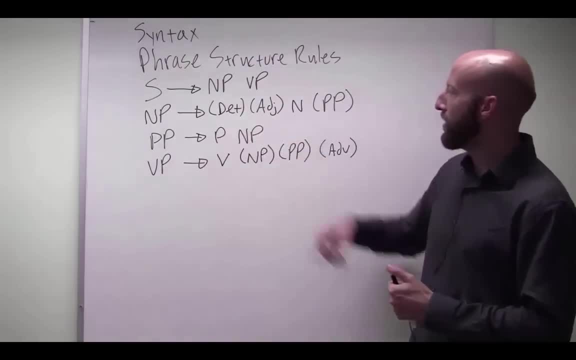 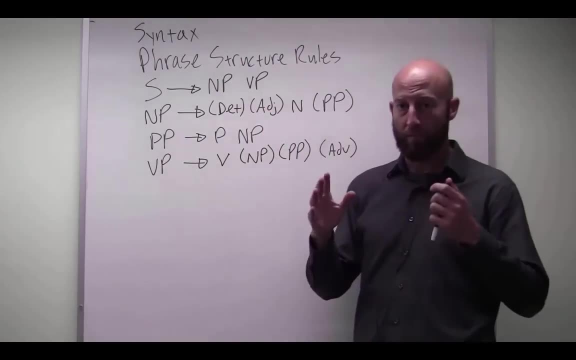 but that's technically true. However, you'll notice that these parentheses are around things like determiners, adjectives and a prepositional phrase that we'll get to in a second. The parentheses mean that they are optional. You don't need them, but you've got to have them. 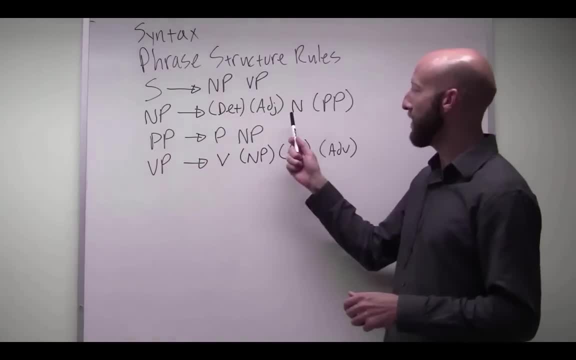 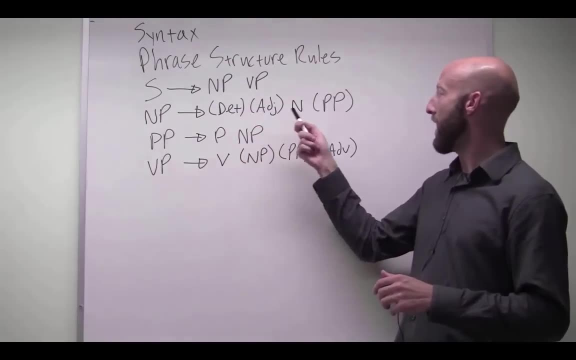 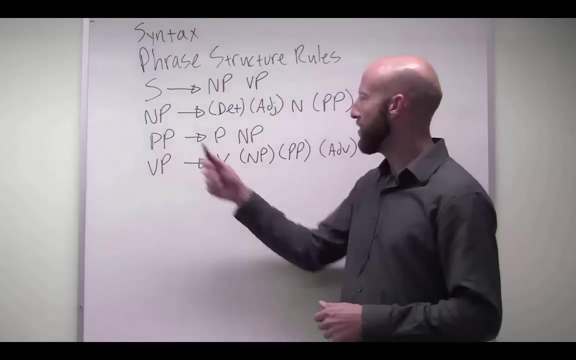 You'll very often get them in noun phrases. So you could have something like just house, That could be a noun phrase, But it could also be something like the red house or the red house on the corner as a prepositional phrase. So a prepositional phrase. then you have to have a preposition and a noun phrase. 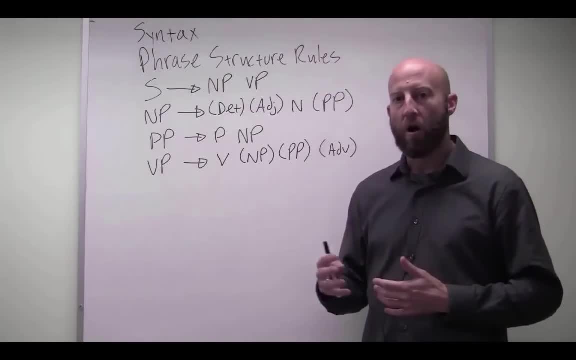 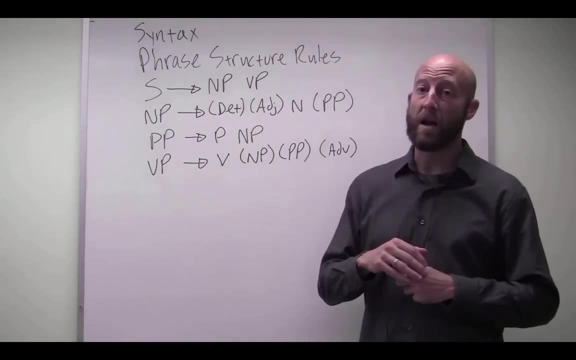 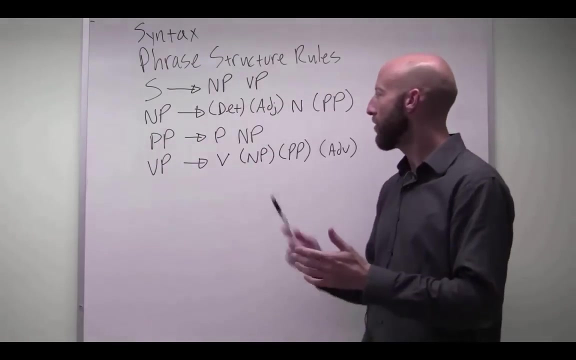 So again, that preposition to near, by, across from. those are all examples of prepositional phrases, All examples of prepositions in English, but they always come with some sort of noun phrase. So near the pool, by the mountain, the pool, the mountain, those are examples of noun phrases in English.